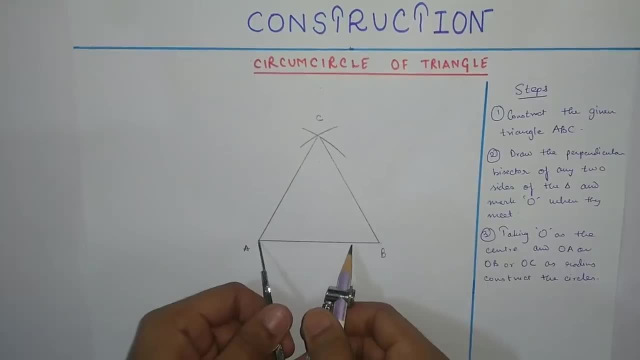 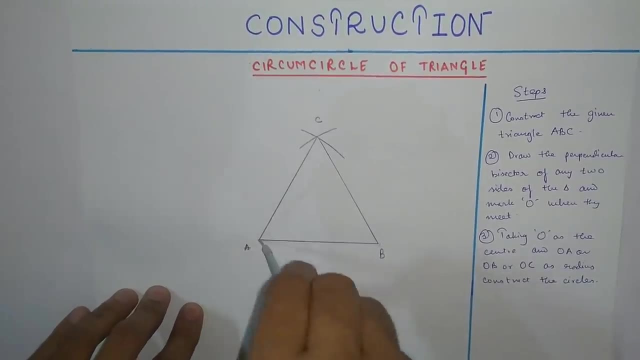 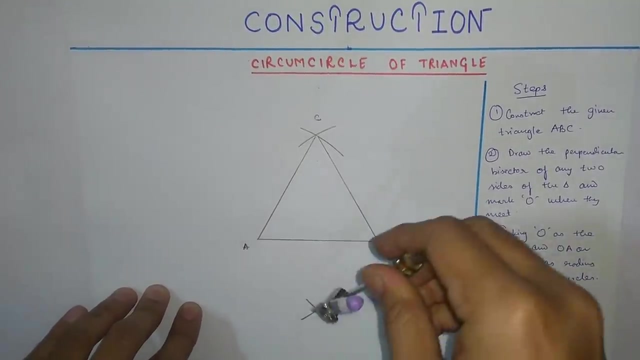 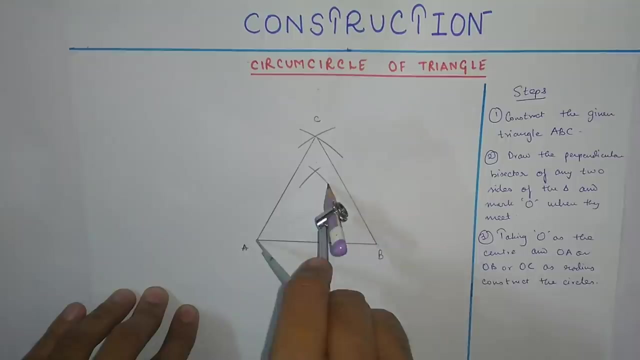 Well, take a compass and more than half the distance or half the length of the line, make an arc over here, an arc over here, similarly over here and over here, to join these two points. So this is the perpendicular bisector of any two sides of the triangle. 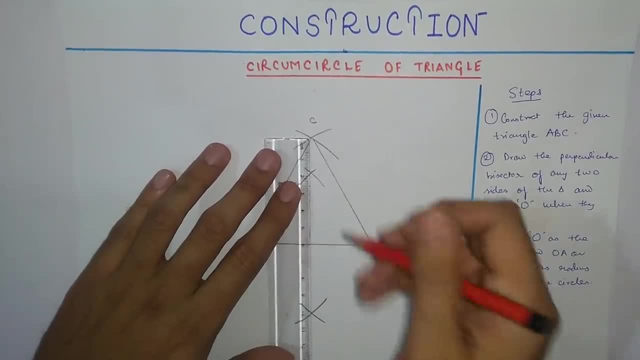 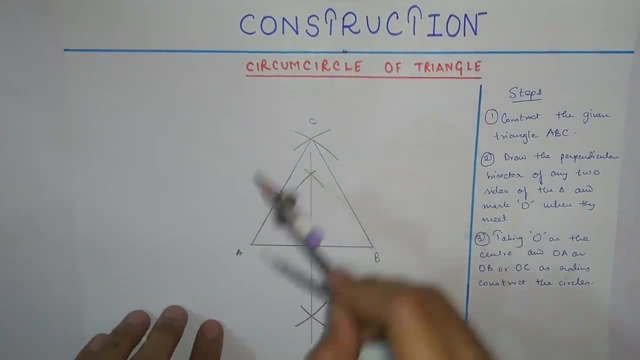 Now step number 3 is you have to draw the perpendicular bisector of any two sides of the triangle. So this is the first perpendicular bisector. you have to make another perpendicular bisector. I will take this side, one over here, one over here, one from here and here. 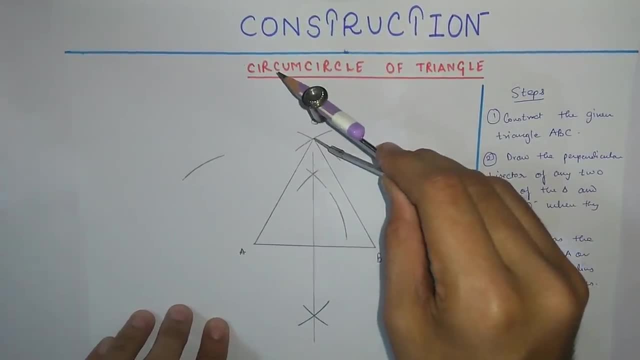 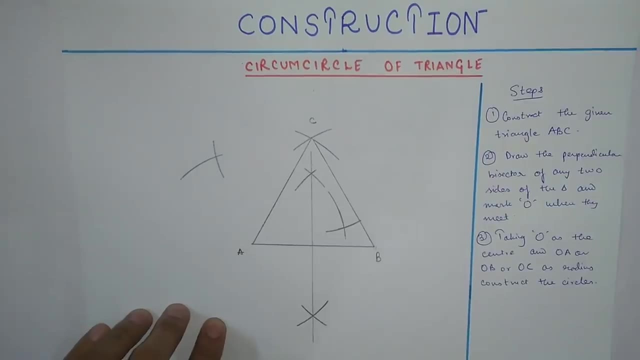 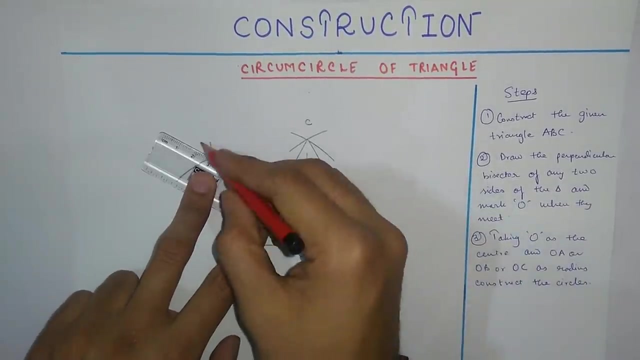 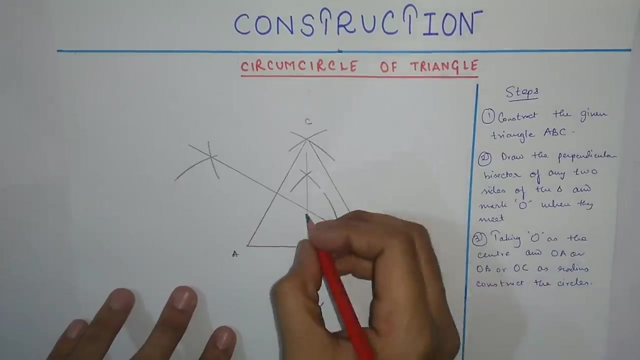 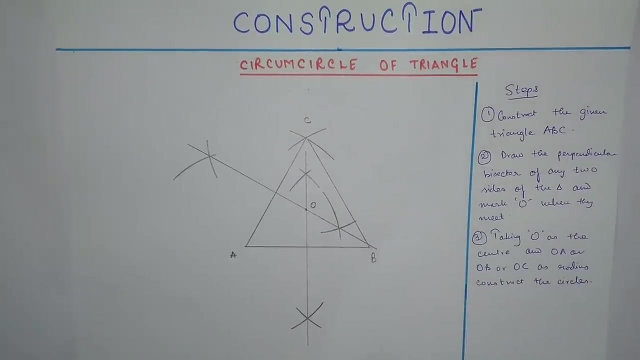 You have to join these two points. So this is the first perpendicular bisector. Okay, Now you have to mark O where they meet. So this is where they meet. mark it as O. Now, what is the third and final step? Taking O as the centre and OA or OB or OC as the radius, construct the circle. 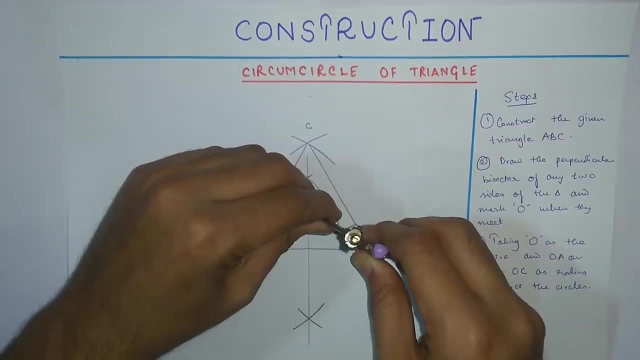 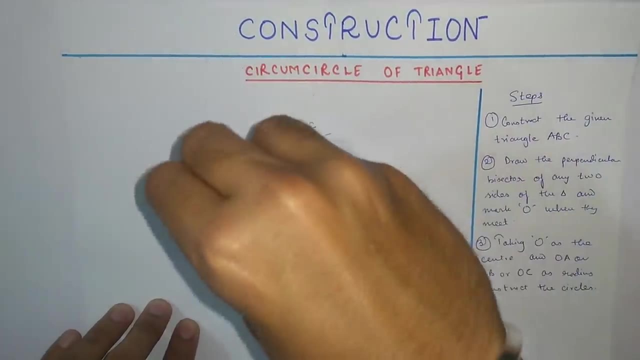 So this will be the centre of the circle. This over here will be the radius. So, as you can see, this is the centre of the circle. This over here will be the radius. So this will be the centre of the circle. So, as you can see, I will construct the circle. 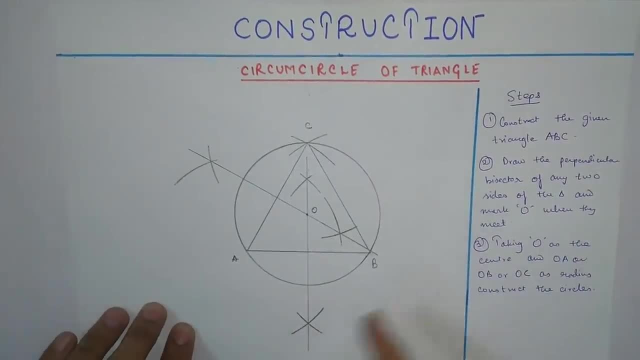 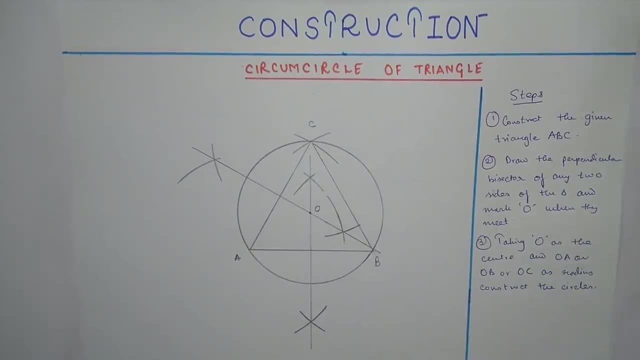 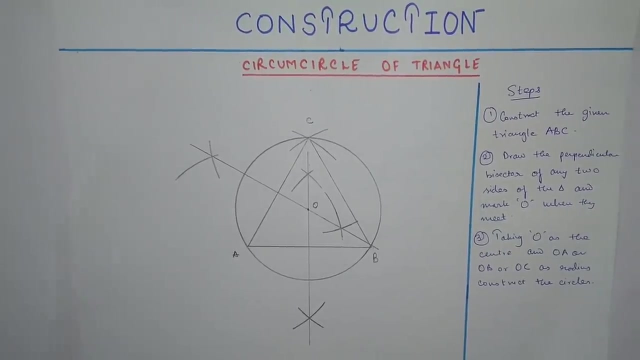 This is a perfect circum circle of the triangle. So this is the required circle. with OB as the radius, We are done with the circum circle of a triangle. Now this triangle can come or cannot come. You can, you will be given other type of triangles, but constructing a circum circle is similar. 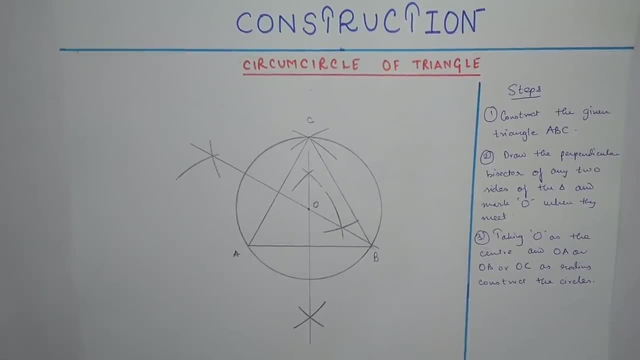 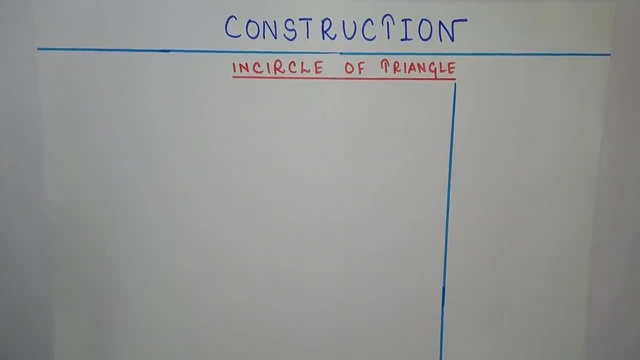 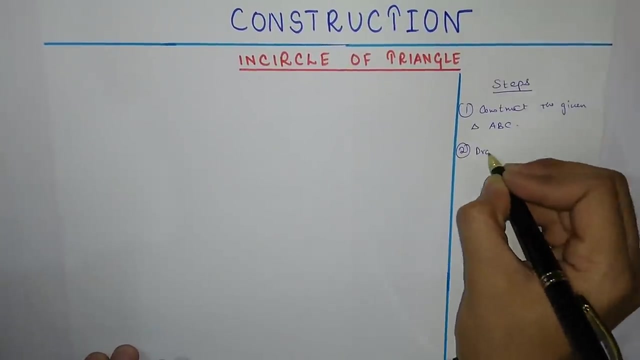 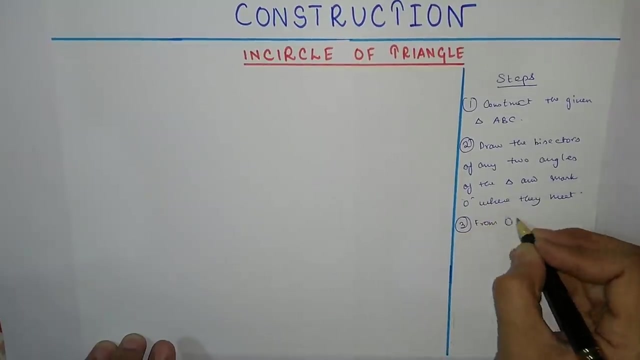 to this, You have to find any two perpendicular bisector of any two sides. Join them. Join them and construct the circle. So we are done with this. Moving on to the construction of incircle, of a triangle, Let's write the steps first. 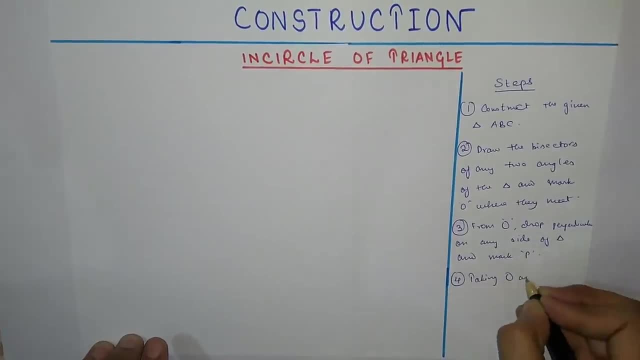 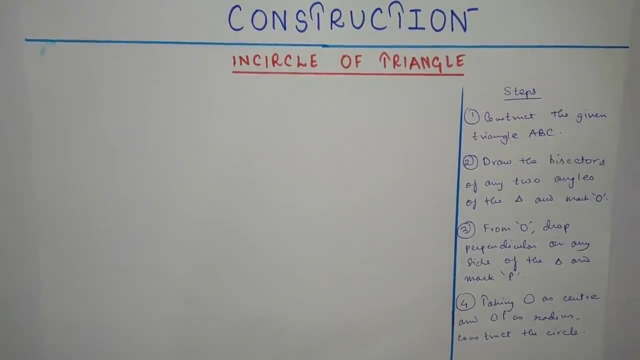 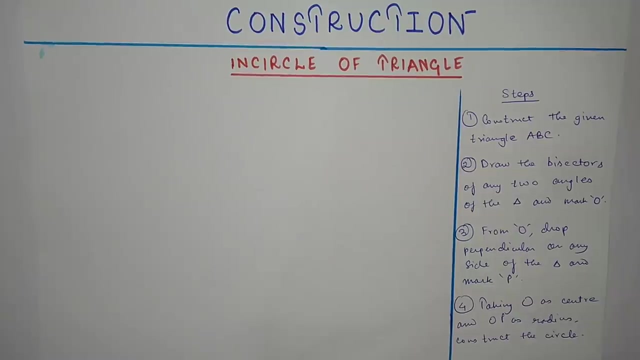 Let's write the steps first. So let's write the steps. So let's write the steps first. So let's write the steps first. So we are done writing these steps Now let's start deconstruction. Now. remember one thing: in circle is a bit tough than circumcircle. So go along with me and you will understand it. So I will make an equilateral triangle of side 9 centimeter in this. 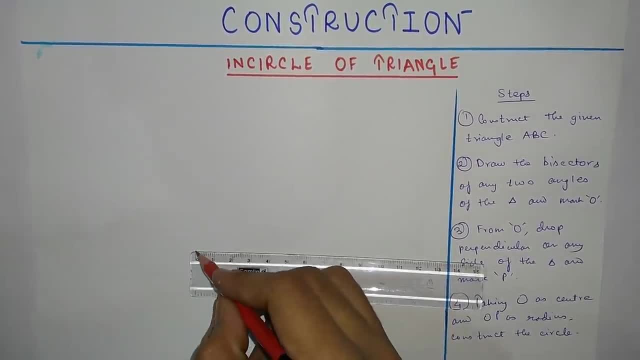 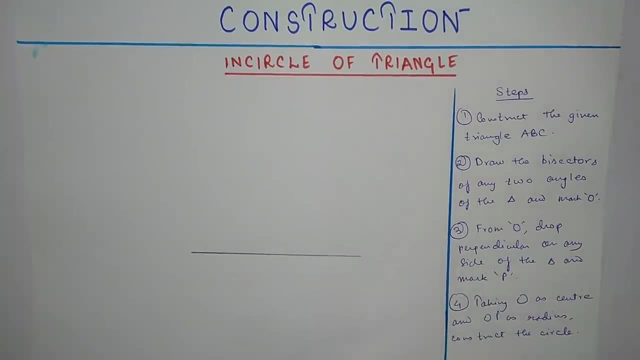 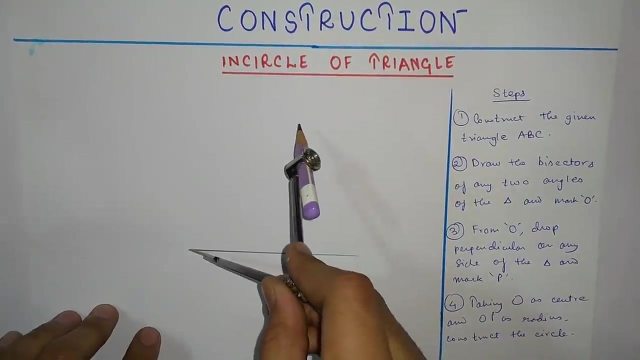 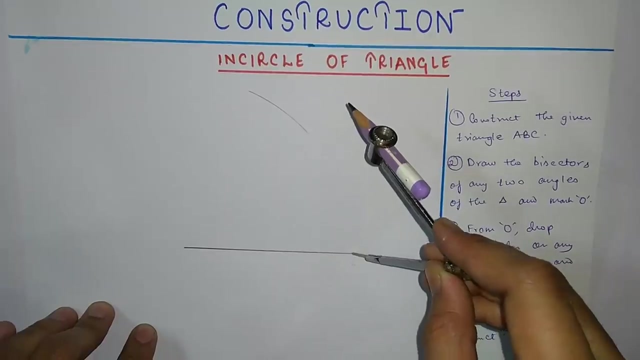 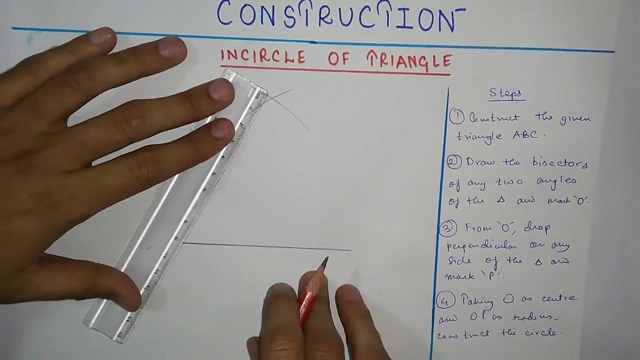 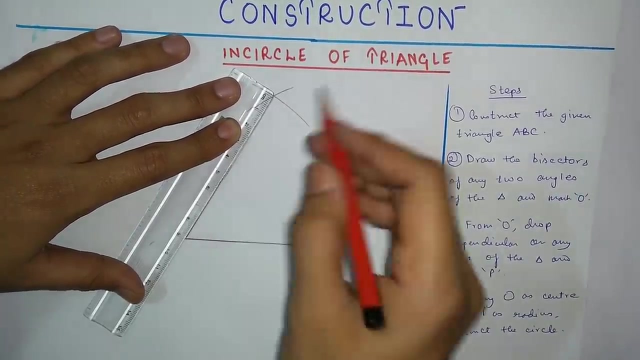 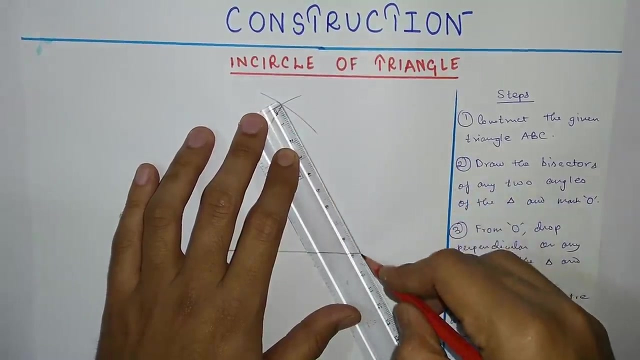 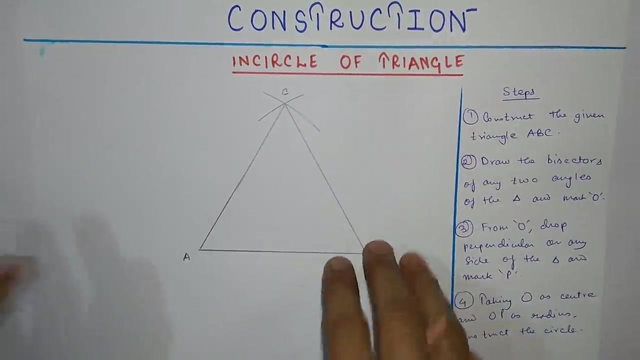 So this is 7,, 8 and this is 9.. Okay, 9 centimeter compass, This is 9.. Now we will just join it. So this is the equilateral triangle. I will mark it ABC, A, B and C. Okay, 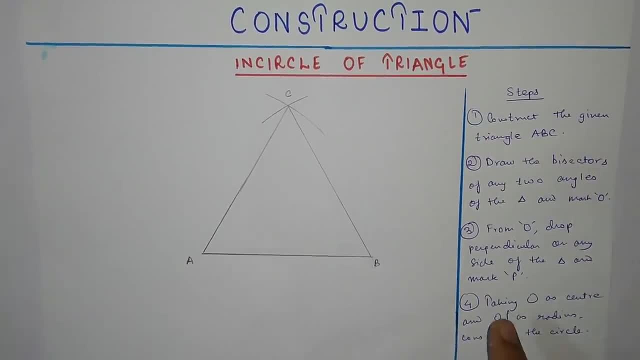 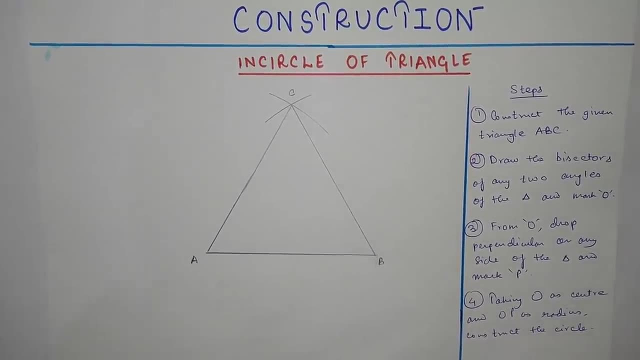 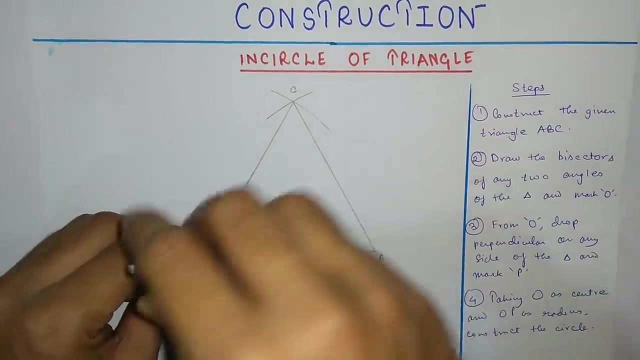 So this was the first step: Construct the given triangle ABC. Now the second step is draw the bisectors of any two angles of the triangle. Okay, how to do that? Compass. This is the angle. This will become a bit big. So over here It is fine. 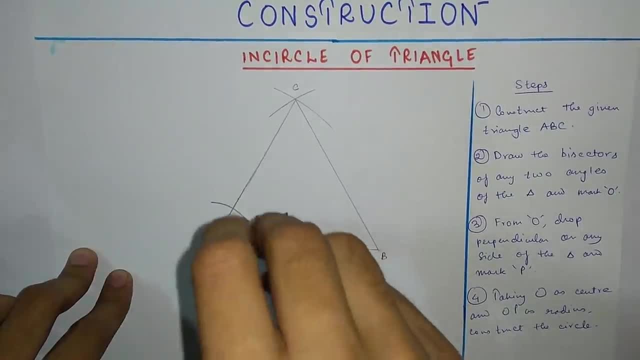 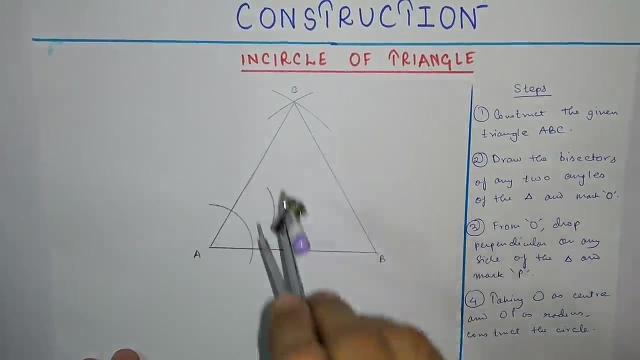 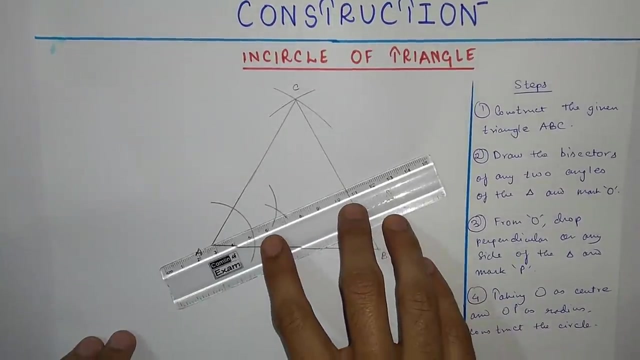 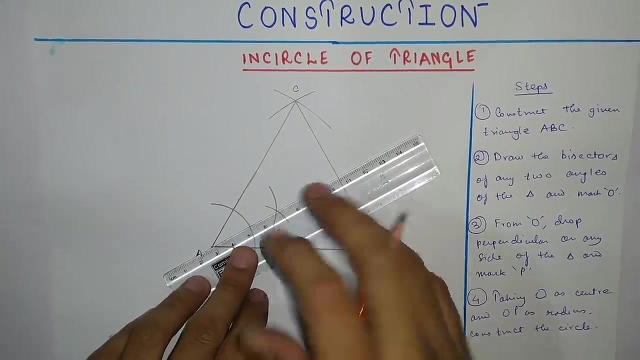 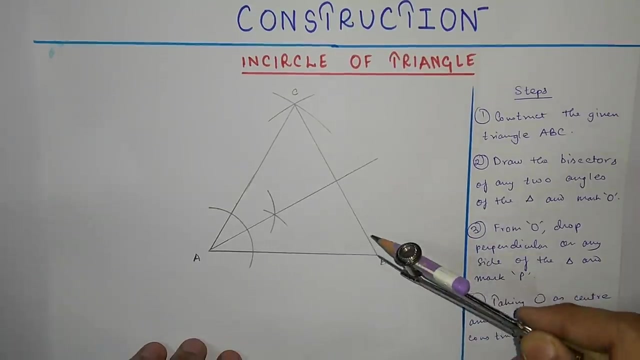 Okay, I will make one arc like this, And then over here and over here. Okay, So this was the first angle bisector of angle A. Okay, I will join it now. We have joined it Now. similarly, we will do this with B. 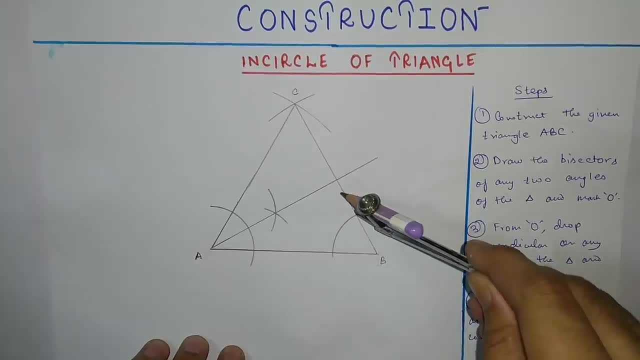 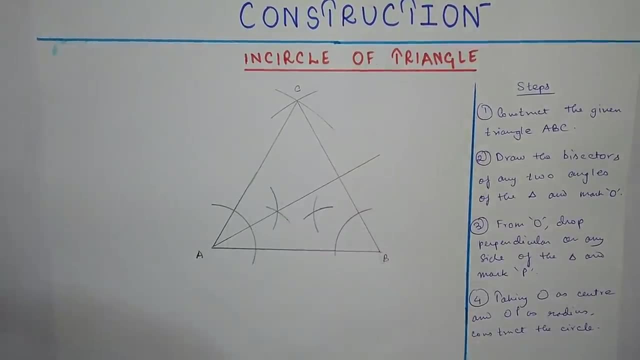 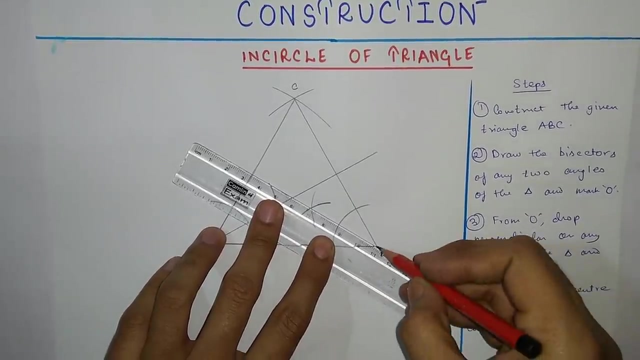 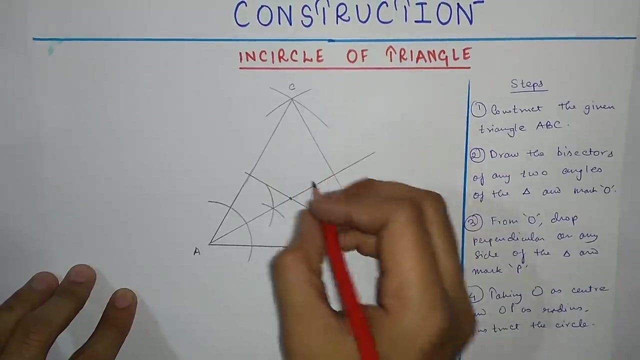 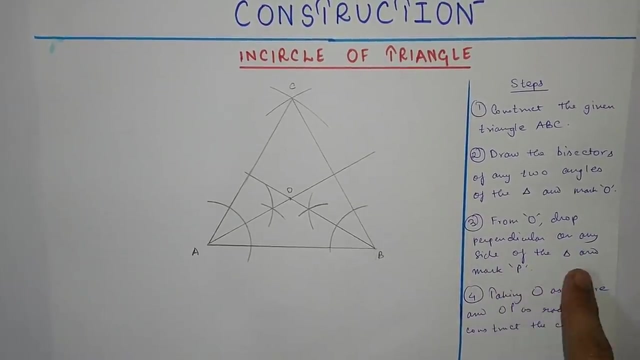 This is B. Okay, This is the angle bisector. We will join and make the line. Okay, This is where they meet. I will mark it. O. Okay. Now the third step is from: O: draw perpendicular on any side of the triangle and mark P.